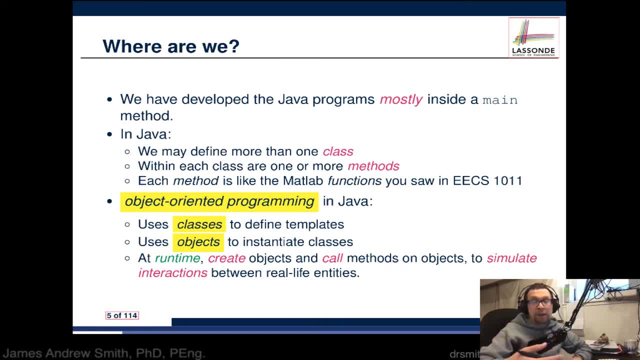 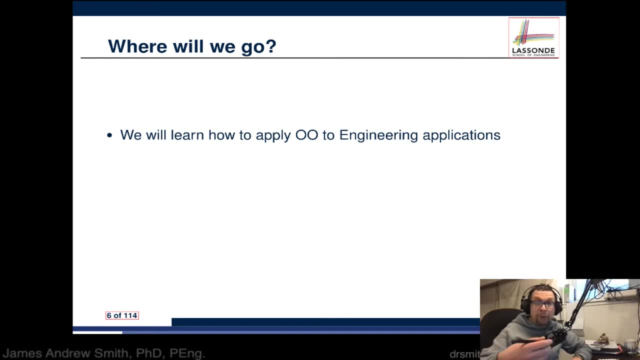 like real world entities: between a dog and a family member, or between you and the cashier at your favorite store, etc. Okay, so where are we going to go with all this? Well, we're going to learn how to apply object-oriented ways, paradigms, to engineering applications. We're going to look 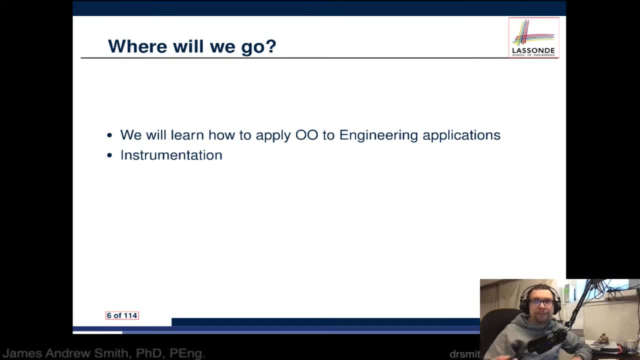 at how that applies to examples of instrumentation. We're going to look at how to apply object-oriented approaches, okay, or mechatronics, or graphical user interfaces. Basically, you know, from the perspective of this course, we're going to be looking at how do you connect your PC Windows. 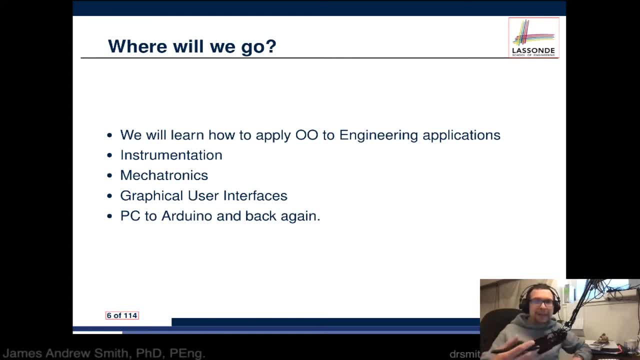 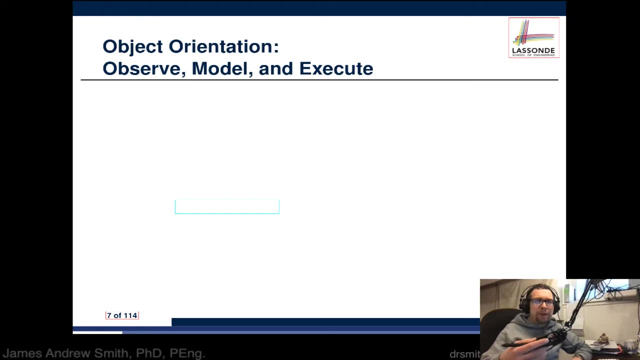 or Mac or whatever, to an Arduino. and then back again, And we're going to be looking at instrumentation, mechatronics and graphical user interfaces from that perspective. okay, How we get that Arduino to talk to your PC, All right. Now, object-oriented approaches, We've got observation. 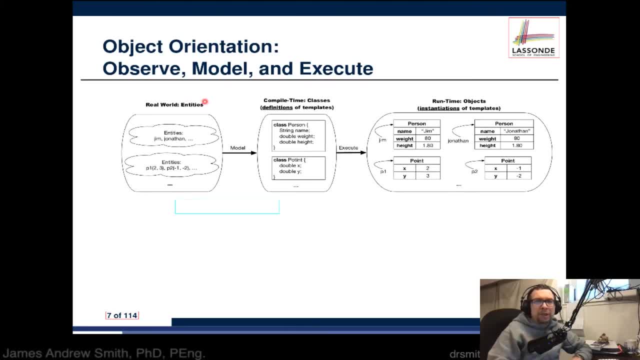 scheduling and execution. So we take a look at sort of in the quote-unquote real world. we have these entities And these entities could be people. They could be like Jim or Shan Yi or Jonathan or Julie. We have entities. They can be numbers and sort of numerical things as well. okay, So 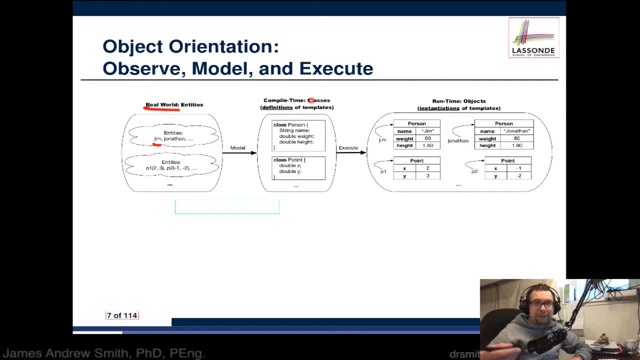 at compile time we have in Java, we have classes, And these are basically definitions of what we're going to be doing. So we're going to be looking at how we're going to be doing this And we're going to be looking at how we're going to be doing this And we're going to be looking at. 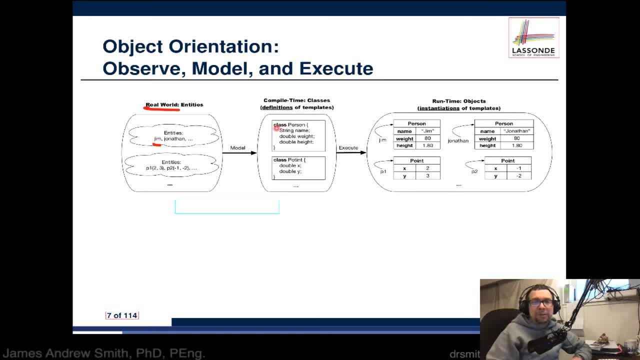 templates, plans, okay, And so you might see the word class, And then that class has a name associated with like person And in it it's got variables like a name or a weight or a height, okay, Or in this case that should actually be point not pot int, Okay, but another class. 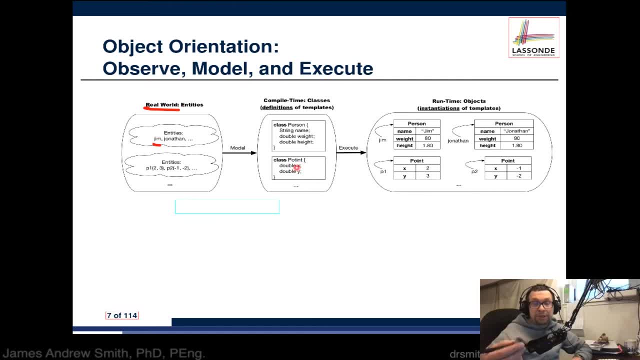 a class point and that has double precision floating point characteristics inside, okay, And one of these would be the variable x and the other one would be the variable y, And then at runtime. so once we've finished writing up our program and we're actually 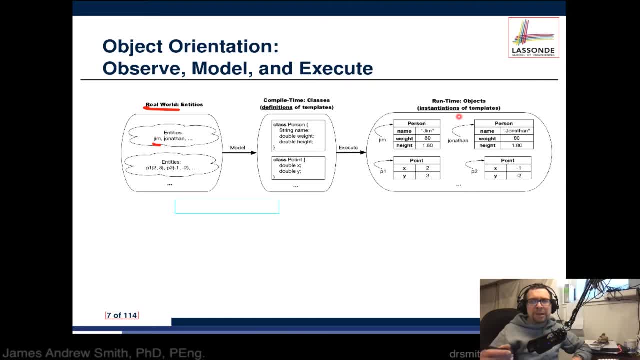 running it. then we have objects, And these objects are the creations of the plans. You're taking the plan and you're making it to actually something, You're instantiating them, okay, And so you would have a person, and that person would have a name Jim, and would weigh 80 kilograms. 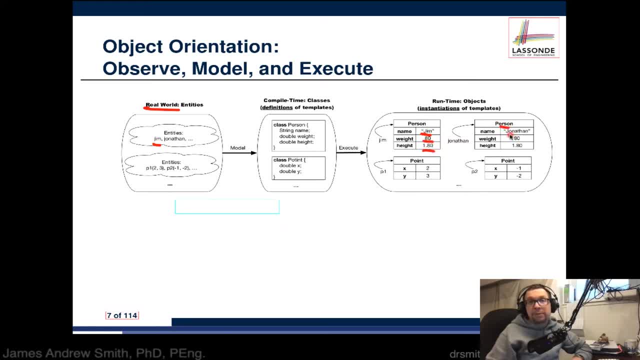 and would have a height of 1.8 meters. And then you have another person. That other person could be Jonathan, with a, you know, with those characteristics as well. You could also have some sort of arbitrary thing, an object called P1, okay, of type point, and it has these numeric. 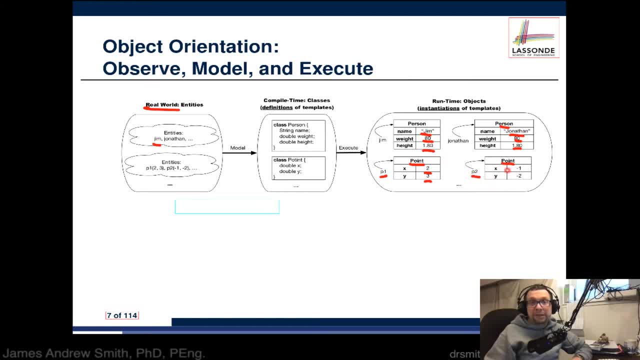 characteristics. We could have another object called P2, of class or type point. okay, with those numerical characteristics inside. Now there's some tutorial videos that you can sort of click to, and we can make a link to that later as well. okay, that'll walk you through the idea. 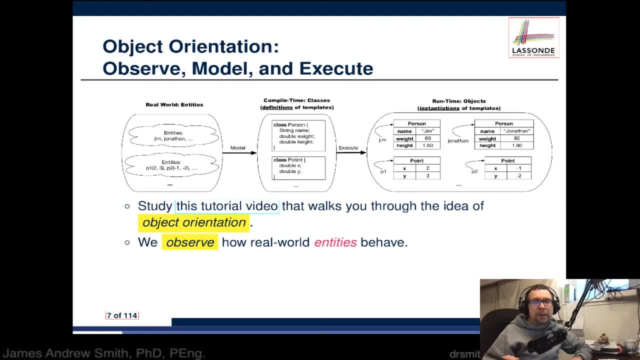 of object-orientedness or object orientation. Now, it's important to point out that this is a programming paradigm and it's based on observations of real-world entities, objects and things and people and that sort of thing, And we model the attributes and the behaviors. 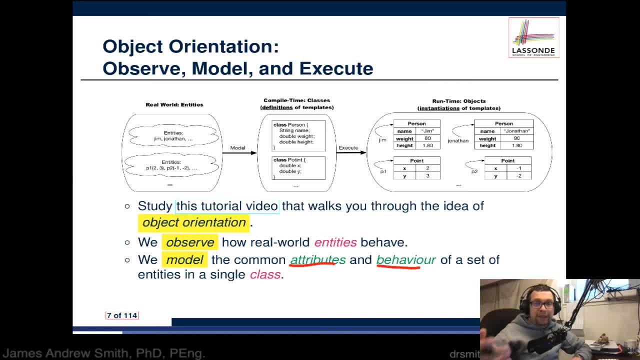 okay that we see in real-world things as a set of entities in a single class. So basically, attributes would be like nouns or adjectives, okay, and behaviors themselves would be more along the lines of verbs- okay. So we execute the program by creating. 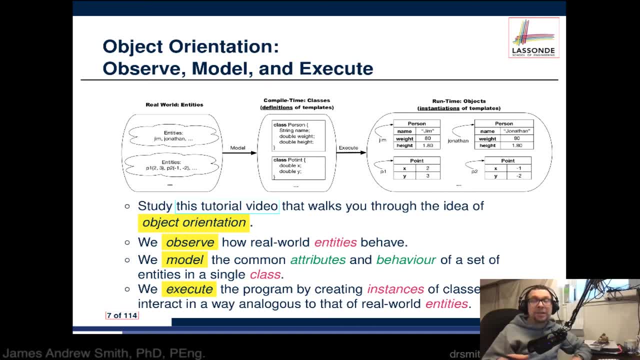 instances of classes which interact in a way that is analogous to these real-world entities. So really, object-oriented programming is based on, basically a view of the world. okay, and the assumption underlying it is that it's a real-world entity and it's based on a view of the world. 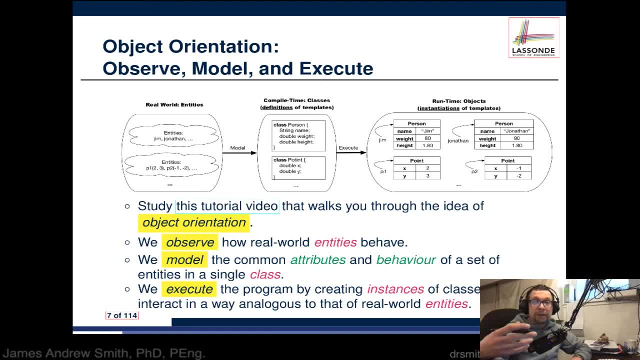 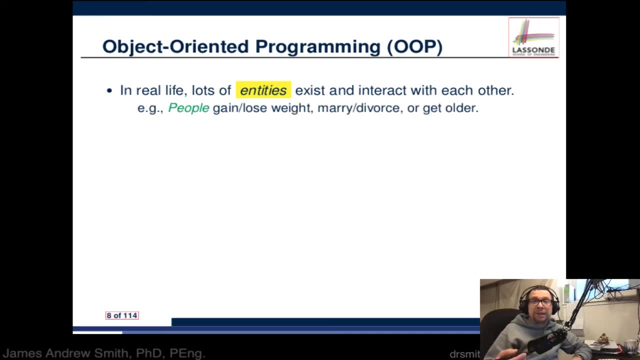 is that? well, if it works in the real-world, then we can, and it's intuitive for people to understand, and maybe we can create programs that are just as intuitive and work in similar ways. All right, so in real life, lots of entities exist and interact with one another. So for